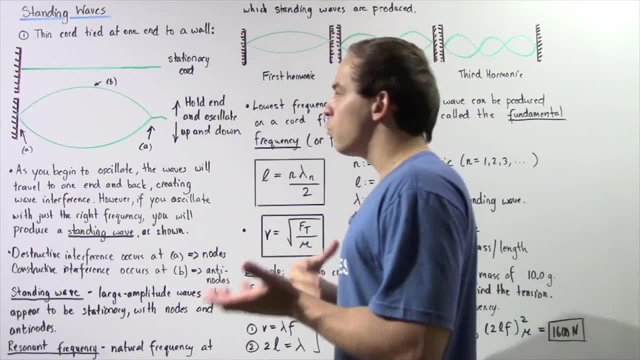 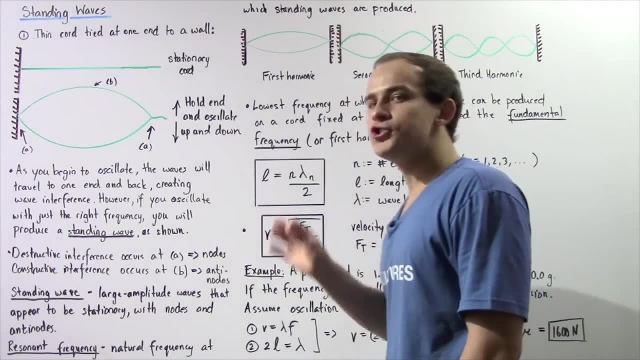 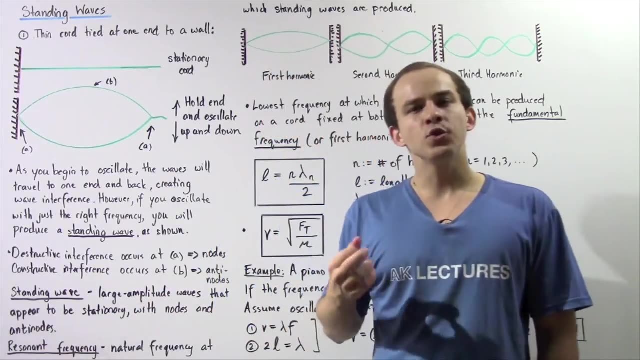 So what we're essentially creating is a jumble of waves that will interfere with one another. Now, if we oscillate our cord at just the right frequency, called the natural frequency or the resonant frequency, we create a wave that is called a standing wave. Now, a standing wave. 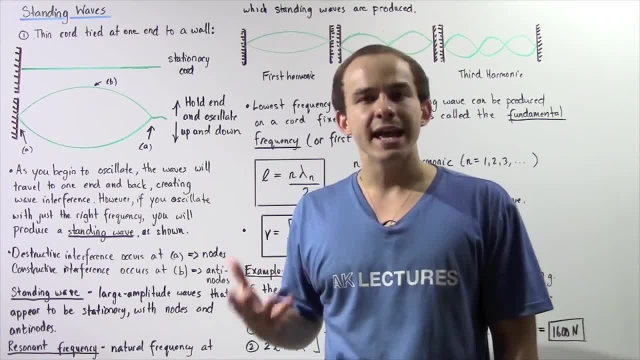 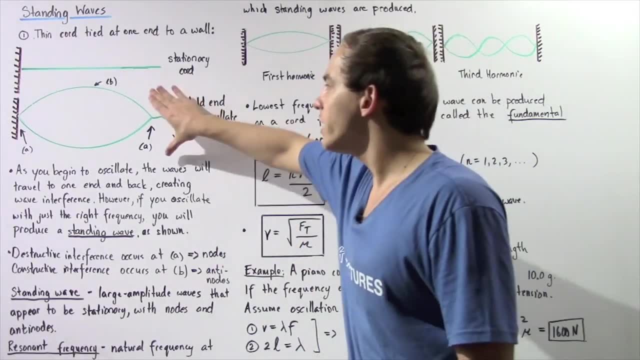 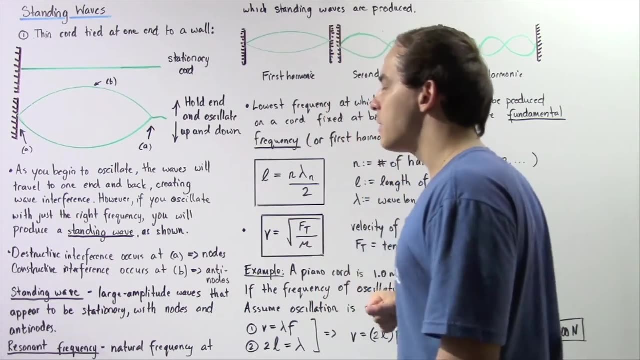 is given that name because it appears to be standing, It appears to be stationary, even though it's actually moving back and forth. So this is one example of a standing wave where, to the eye, our wave will appear to have this shape, but the wave actually is moving back and forth. 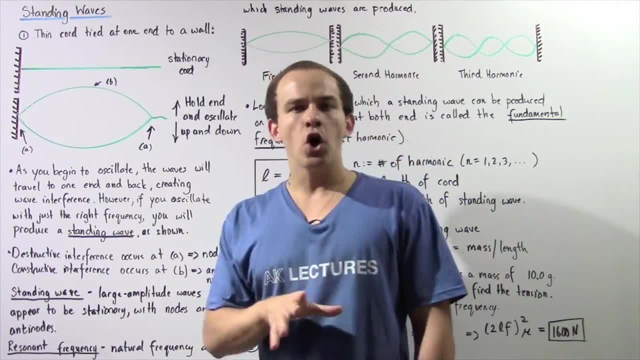 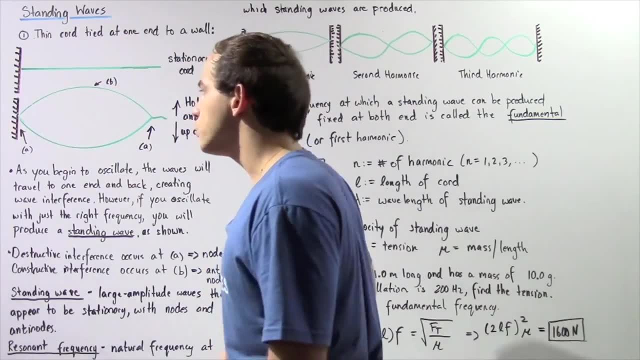 Now, if we take a standing wave, and we take a standing wave, we create a jumble of waves that are propagating back and forth. Now, any given standing wave has regions called nodes and anti-nodes. So these are our anti-nodes, shown by B, and these are our nodes, shown by A. A node is: 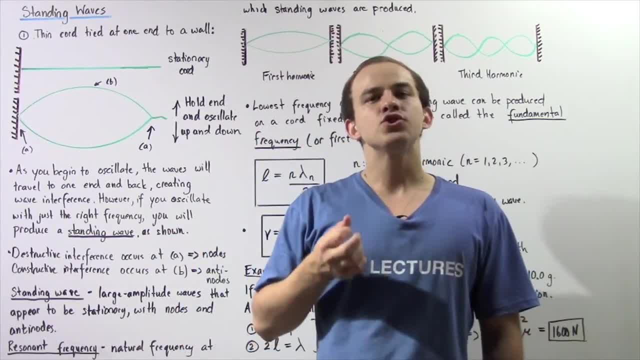 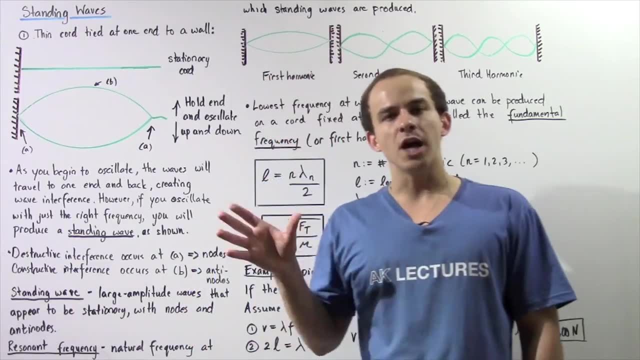 essentially a region on our standing wave where destructive interference takes place. In other words, if we take the algebraic sum of our displacements, of our individual waves that are found propagating back and forth, our displacements will be the same as the displacements of our 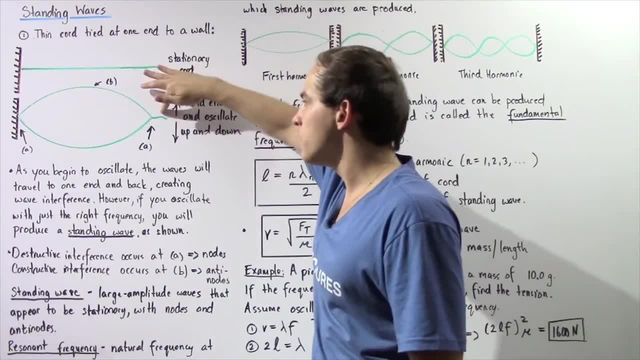 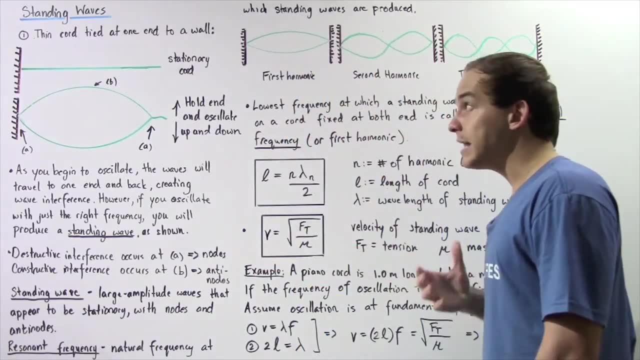 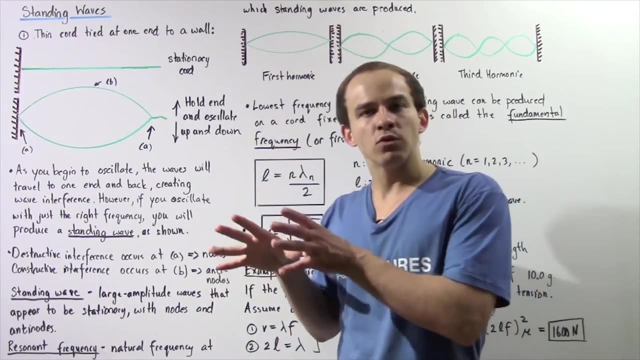 nodes. So the displacement at the node will sum up to zero, And that's exactly why our displacement at point A and point A are zero. On the other hand, at point B we have constructive interference taking place, which essentially means that that will be our location of maximum displacement. So 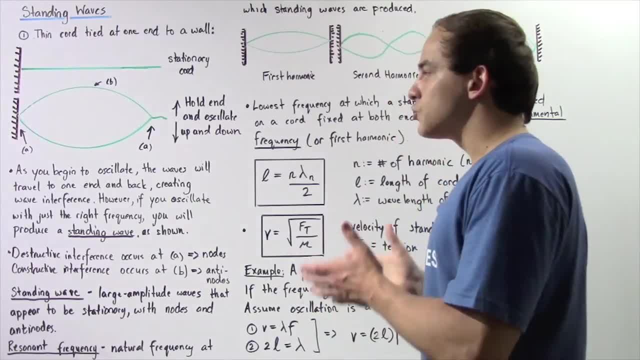 once again: as you begin to oscillate, the waves will travel to one end and back, creating wave interference, a jumble of waves that are propagating back and forth. So if we take a standing wave, we have random amorphous waves in these regions. Although thisC relates to the perspective D, 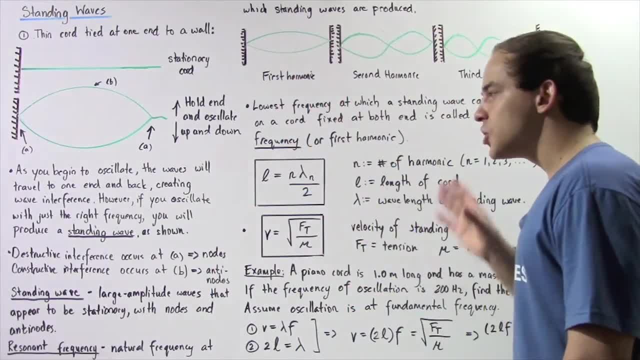 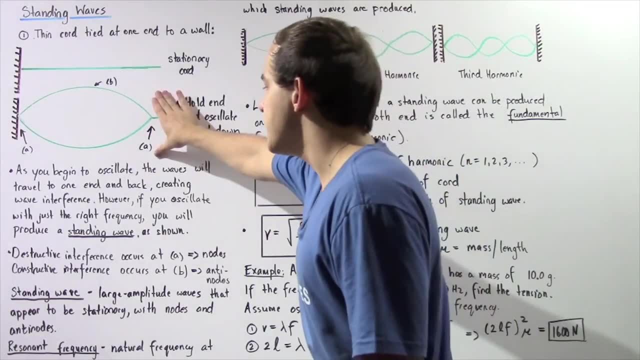 of the programming method that is set in this diagram. However, if you oscillate the frequency of the chord with just the right frequency, known as the resonant frequency, you will produce a standing wave, as shown in this diagram. This standing wave will also have regions called. 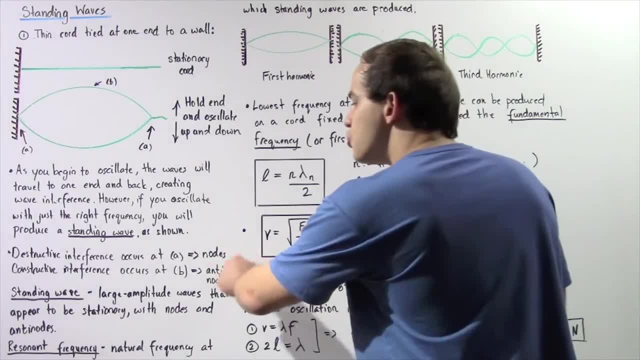 destructive regions where destructive interference takes place, And those are known as nodes, And our constructive interference locations are known as Anit Snodes. So weska use a standing wave as a determiner. where destructive interference, inflammation is achieved even at horizontal times. Hence our routes are donde negative Hessian waves. we have a droite movement of waves in which an anterior historic destructive wave with mutual descending weight to always make not excessive interference. This looks toма like this diagram Once the derivative wave of a wave here is selected for judging. 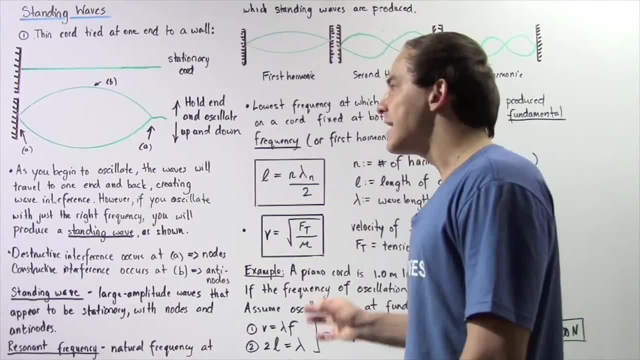 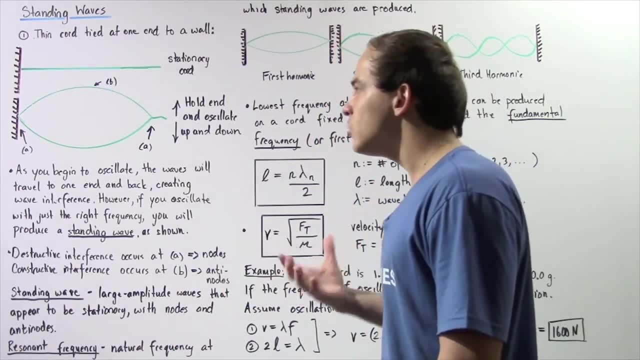 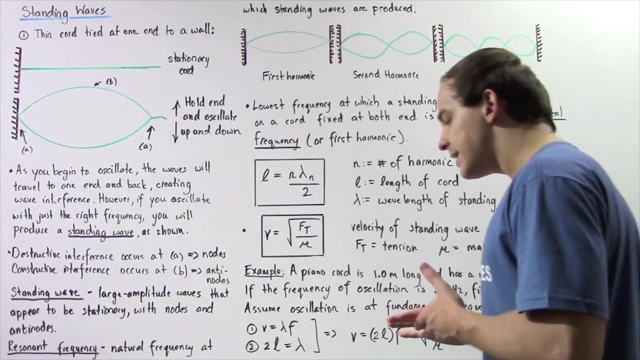 wave is essentially a large amplitude wave that appears to be stationary and has regions called nodes and anti-nodes, And frequencies called resonant frequencies, produces our standing waves. Now, technically speaking, we could have as many standing waves as we want, So the first, 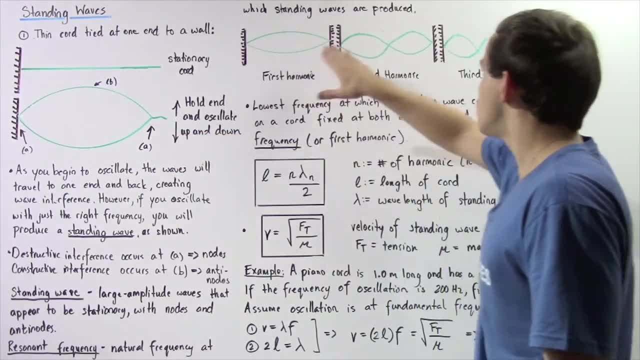 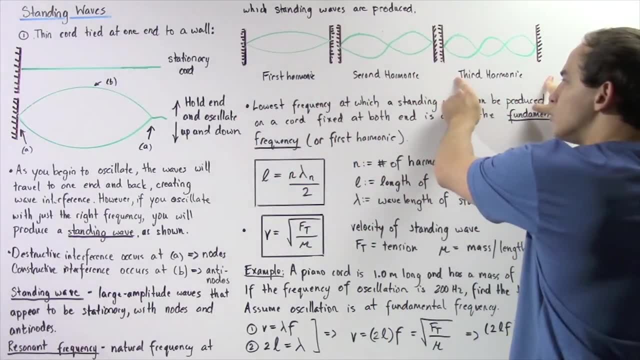 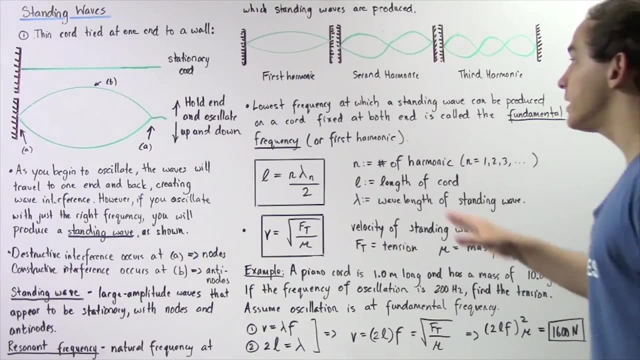 three standing waves for the following diagram are shown in this diagram. So we have our first standing wave, the second standing wave, the next standing wave. Now, the lowest frequency at which a standing wave can be produced on a chord that is fixed at both ends as shown is called a. 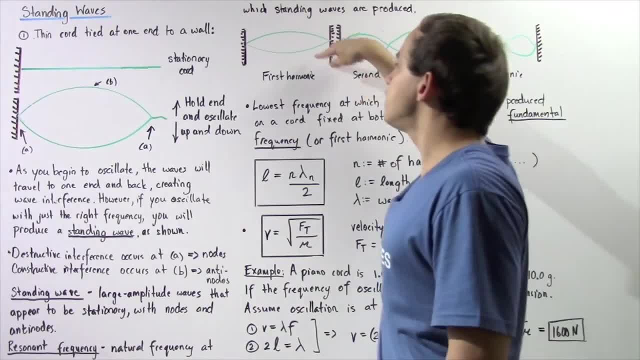 fundamental frequency, or also known as the first harmonic. The next frequency is called the second fundamental frequency, or also known as a third harmonic. The next frequency cannot be determined on a spiral in any way and must be++ plus or plus e- dangerous, So the next level of wrong- or by extreme. 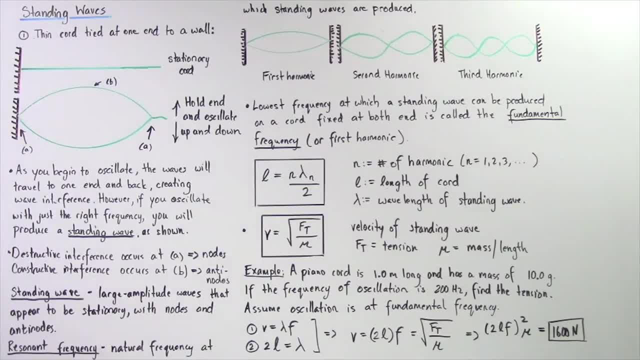 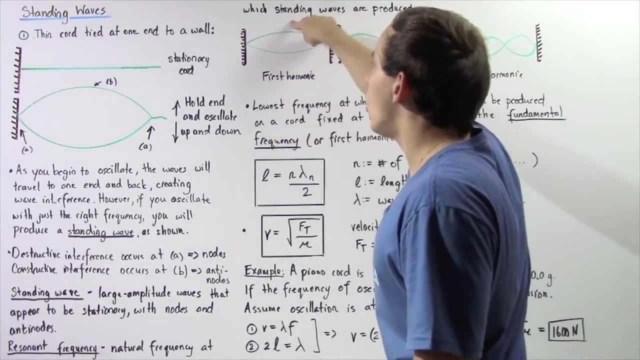 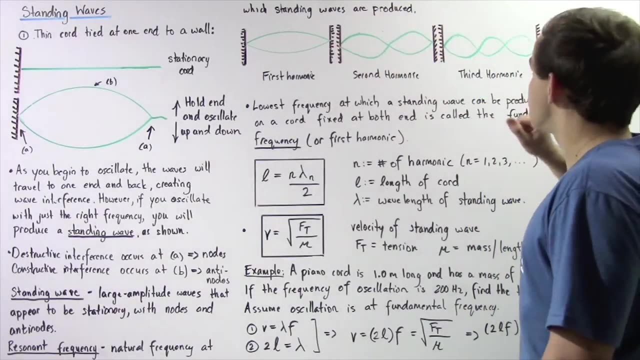 harmonic, the third frequency is called the third harmonic, and so on and so forth. Now notice: our first harmonic in this case has two nodes and one anti-node. The second harmonic has two anti-nodes and one, two, three nodal regions. And the third harmonic has one, two, three, four nodes and one. 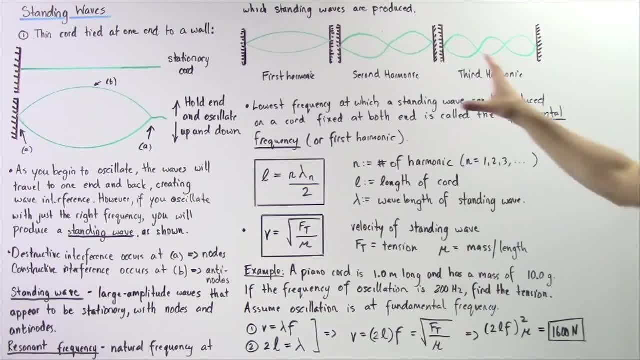 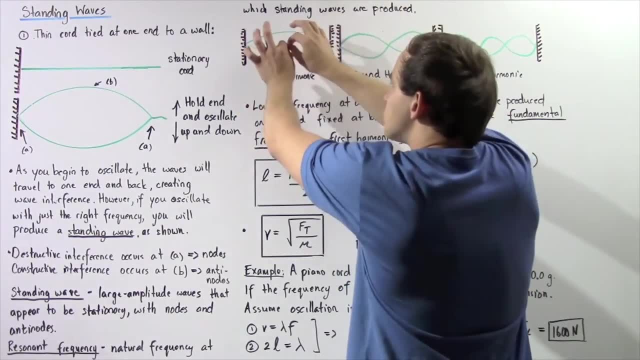 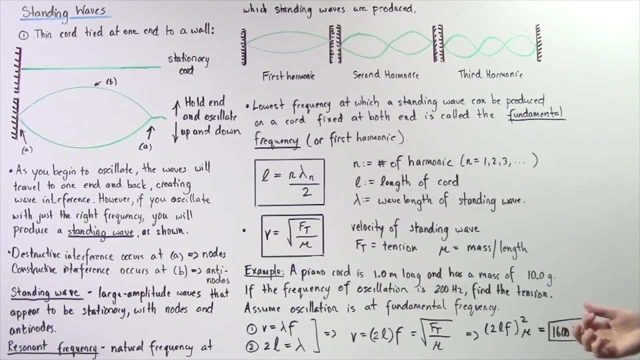 two, three anti-nodes. Now for this particular example, where we have a standing wave that is between two walls, so our string is attached at both ends, is fixed at both ends. we have the following general formula that will give us a relationship between our wavelength of that. 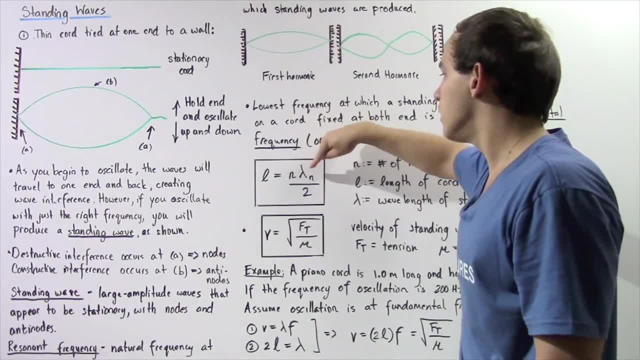 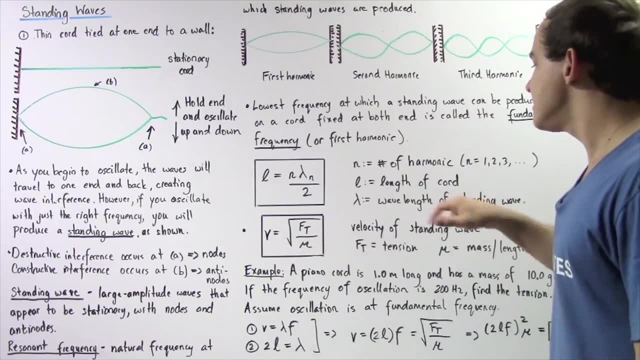 particular standing wave given by this lambda and our L, which is our total wavelength. So after we've got that young formula, we're going to continue to focus on our length of our string or chord. So, once again, L is the length of our chord, our lambda is our. 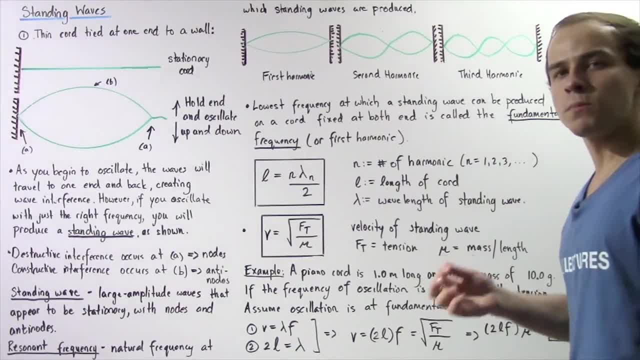 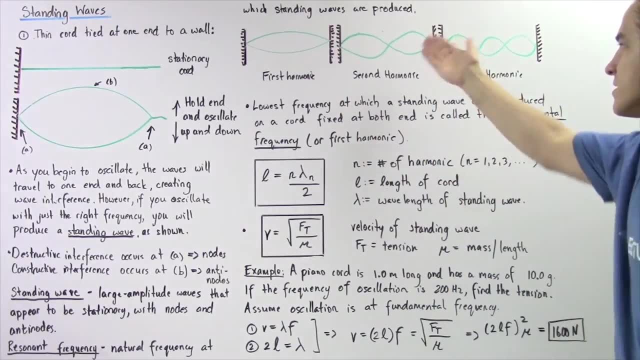 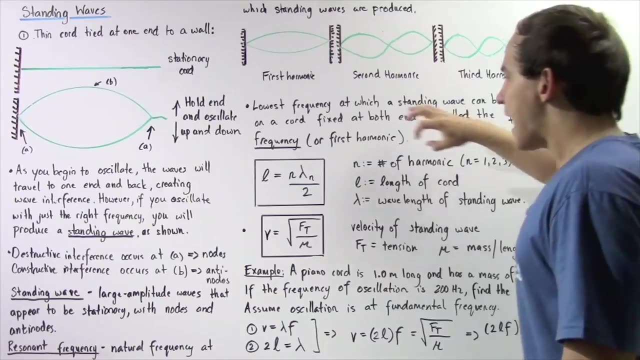 wavelength of the standing wave, and the N simply represents the number of harmonics. So if we're dealing with the first harmonic, N is 1.. If we're dealing with the second harmonic, N is 2, and so on and so forth. So we see that when N is 1, our wavelength for our standing wave is 2 times its. 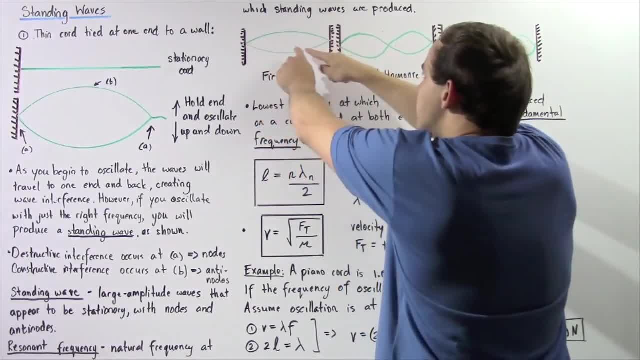 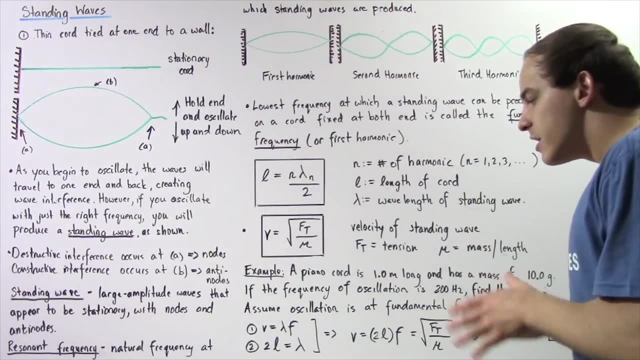 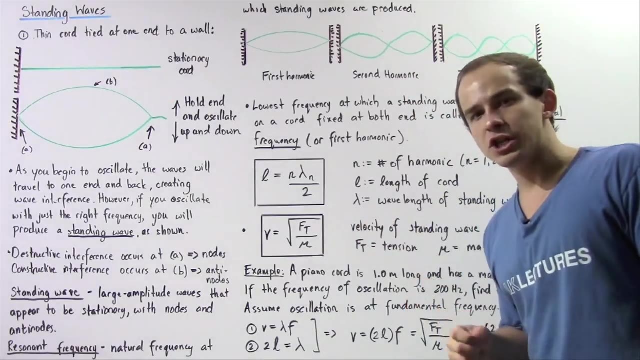 length. So if its length is this entire region, then 2 times this length is the wavelength of our standing wave. Now recall that the velocity of a mechanical wave traveling in a thin chord is given by the following equation: The velocity is equal to the square root of the force in our 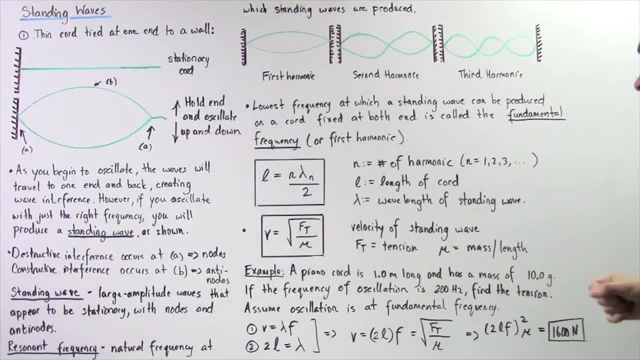 chord divided by our mu, where the mu is simply the mass of the chord divided by the length of our standing wave. So it's a with big S, So it's a control of this applying force. So we have to decreasing it by the square root of the force in our chord, divided by our mu, where the mu is. 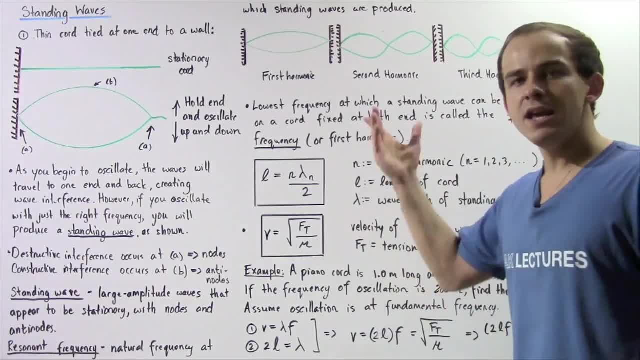 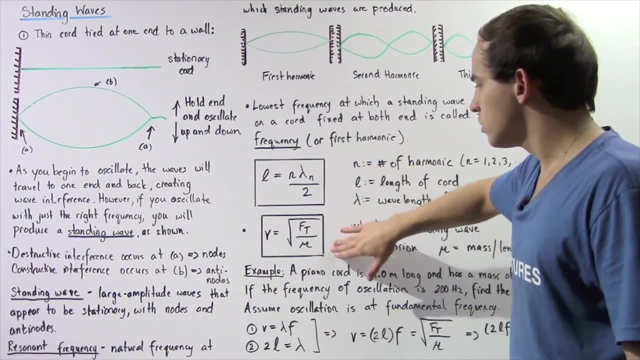 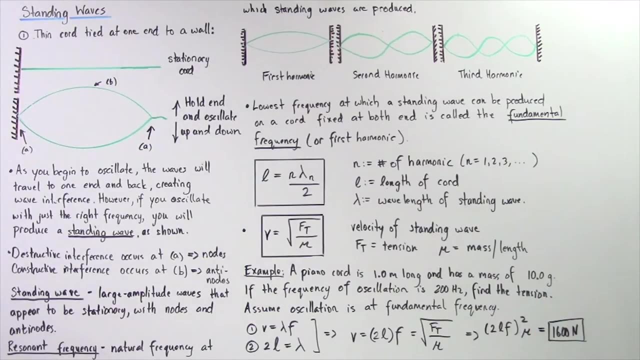 our chord, and this equation gives us the velocity of our particular standing wave. So let's look at the following example in which we're going to utilize these two equations. Let's suppose that a piano chord is 1 meter long and has a mass of 10 grams. 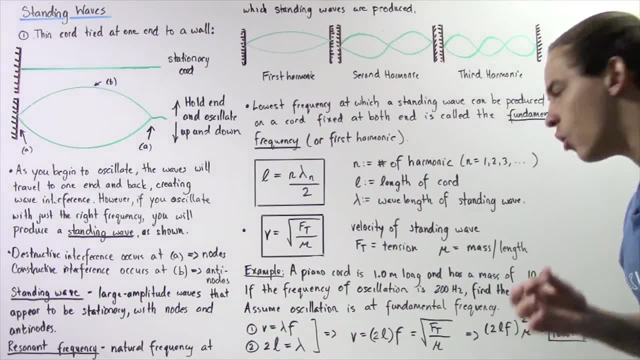 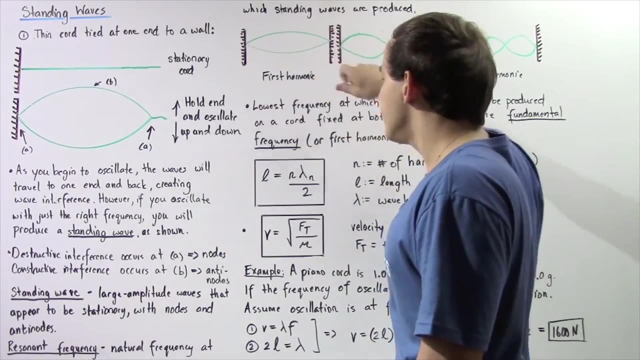 If the frequency of oscillation is given to be 200 hertz, find the tension in our chord, assuming that the oscillation is at fundamental frequency. So once again, fundamental frequency simply means we're dealing with our first harmonic. so that means our n is equal to 1.. 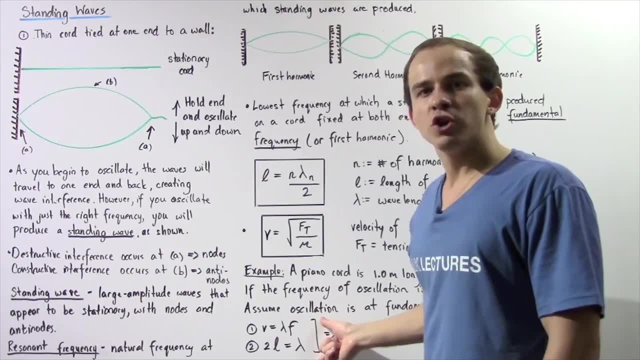 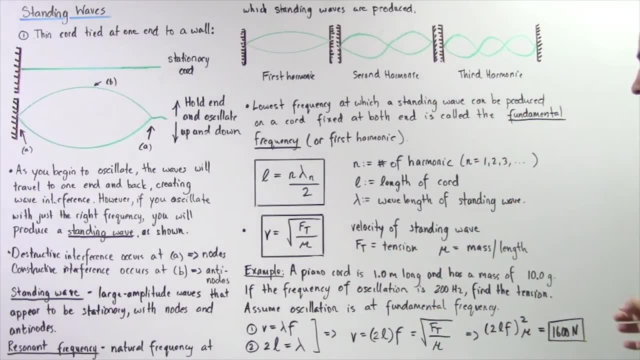 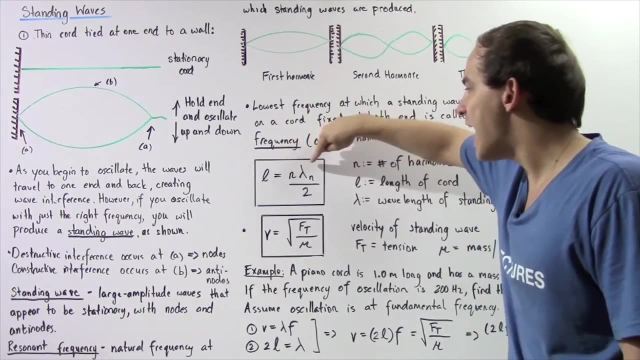 So we want to use the following two equations: Recall that the velocity is equal to the product of the frequency and the wavelength of our standing wave, And we get this equation from this equation, Because our L is equal to 1 times lambda divided by 2.. 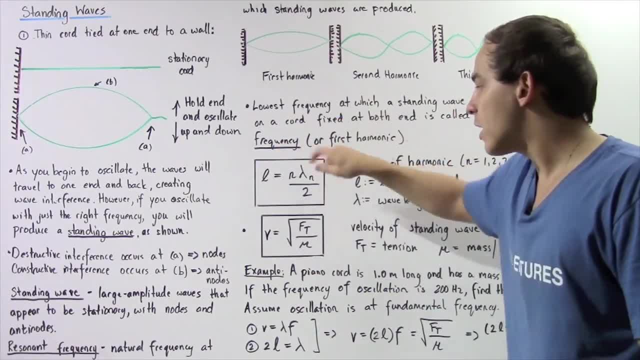 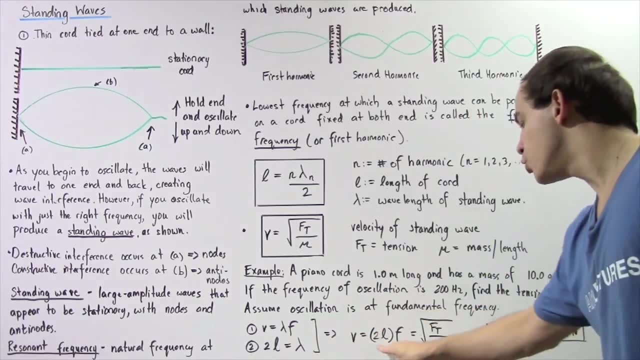 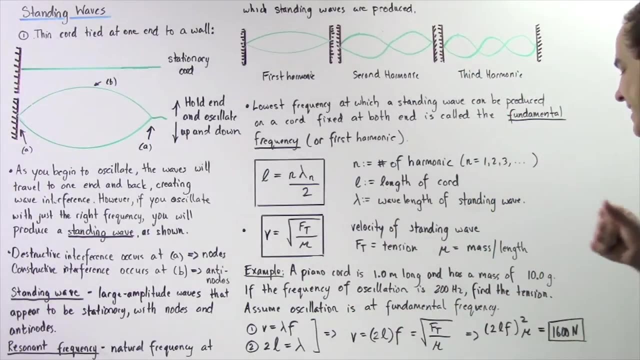 So lambda is simply equal to 2L because our n is 1.. So we essentially want to take 2L and replace our lambda with 2L, And we find that the velocity of our standing wave in that particular chord is equal to.